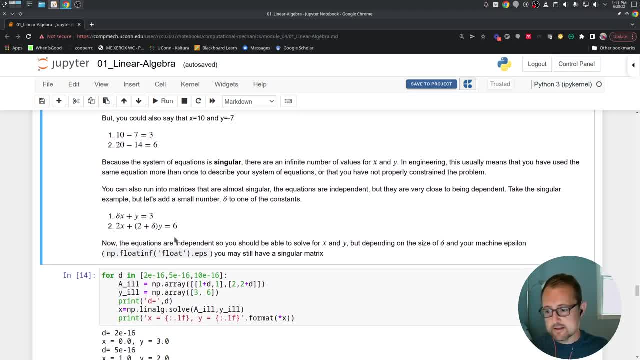 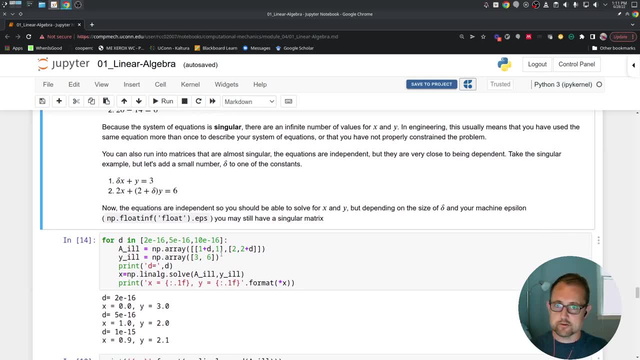 But if you have something that's near singular, technically there's still an answer, like a single answer, but you're going to have trouble discerning what that answer is. So you're introducing error because of those floating point operations. So remember, in a computer, a computer stores numbers as some kind of like 32-bit or 64-bit number. 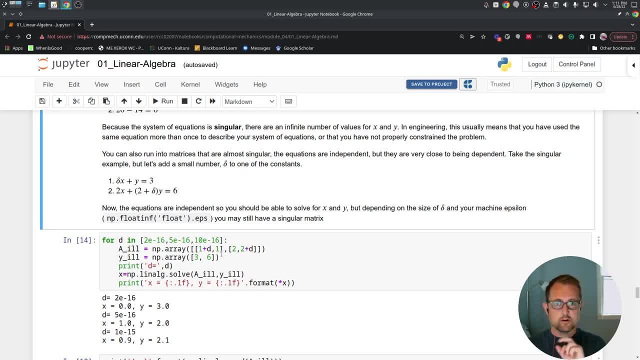 So there's only so many locations where we can either store a 1 or a 0, and we sum those up as powers of one-half. It's either like one-half to the 1, one-half to the 16, to get like 1 over 2 to the 16.. 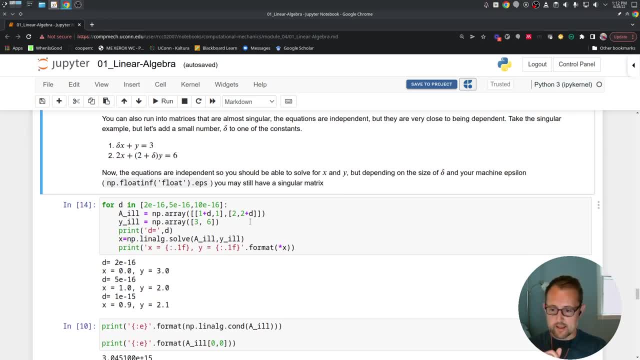 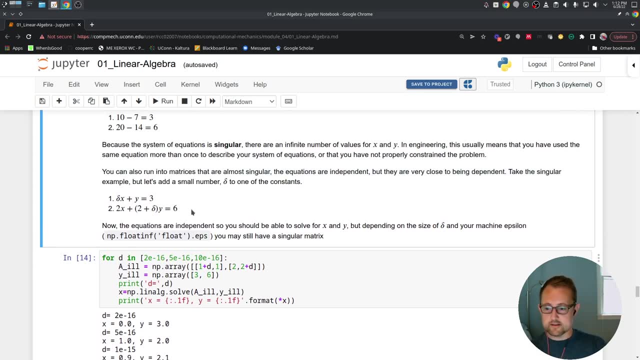 But we're looking- And this is a nice toy example where there is an exact answer but the computer has trouble finding it- depending on what this value of delta is where we're introducing some error And it all comes down to what the condition of that matrix is. 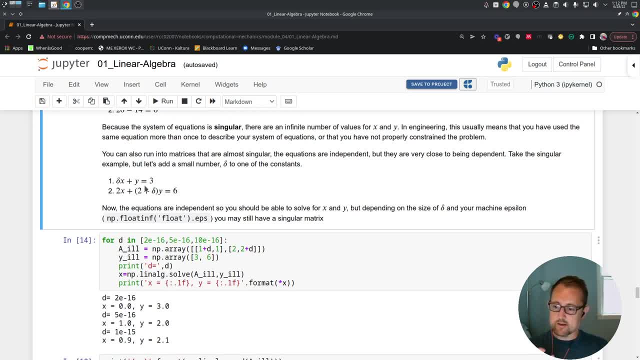 So here I have: delta x plus y equals 3,. 2x plus 2 plus delta y equals 6.. If delta is really small, then these two equations become kind of dependent on each other. We're restating the same kind of equation. 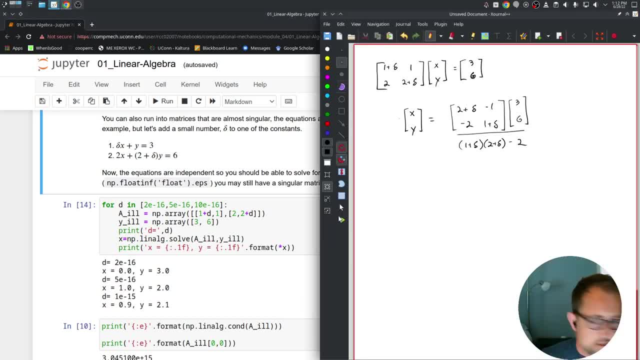 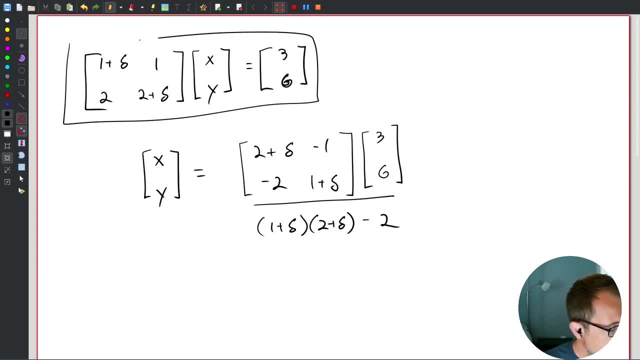 So let's take a look at that. This is the equation that I'm working with. We can blow this up a little bit bigger. Here's the equation that I'm starting with: Right: 1 plus 1 plus delta. Yeah, that's what I want. 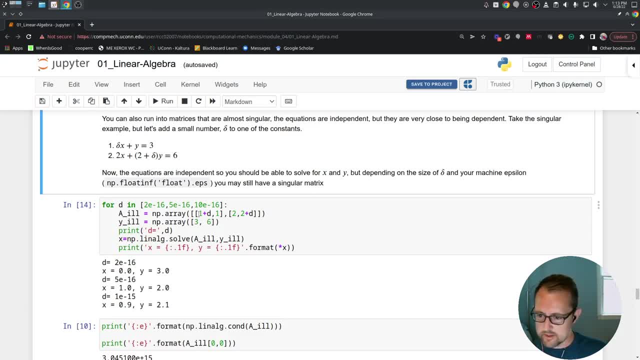 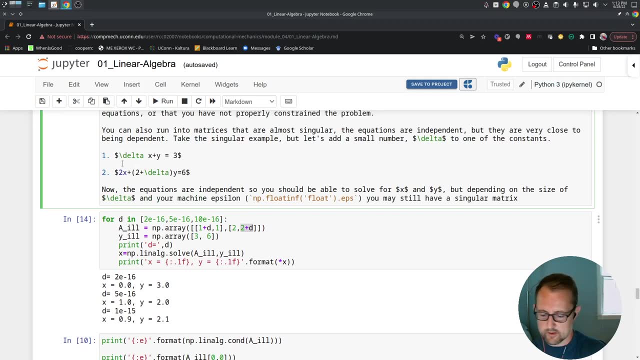 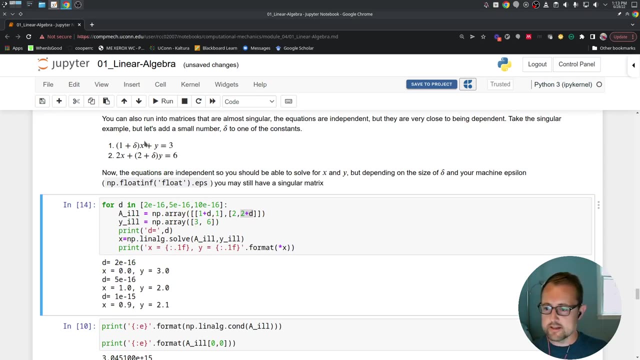 1 plus delta. So there's a typo here: 1 plus delta and 2 plus delta. Because I want: if delta is really small, There we go, Let's do this 1 plus delta, like that. So when delta is really small, these are the same equation, but if it's close to 0, if it's actually 0, then it's the same equation. 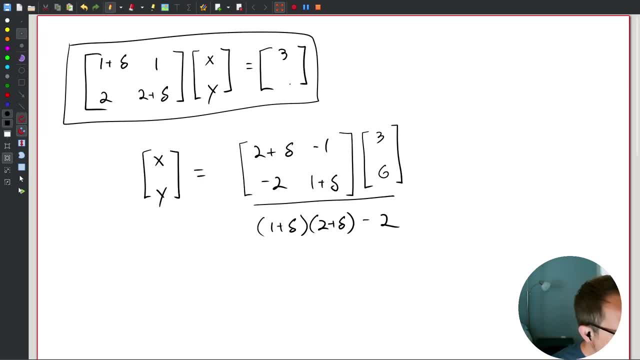 If it's not, Then Okay. So this is restating those two equations in a linear algebra form, So I can invert this matrix. So if I call this A, this is A inverse. This is something that we're not really covering in this class, but 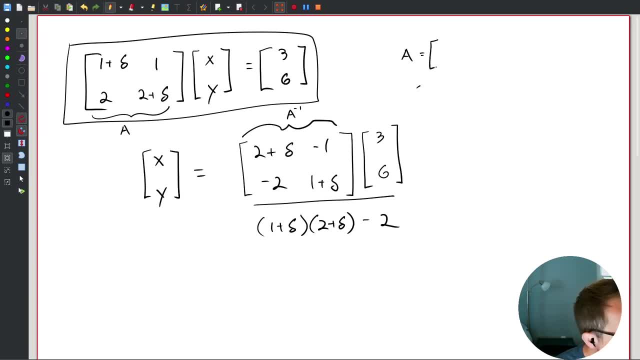 So if A is A, B, C, D A, inverse is D A. So switching those two diagonal elements and then making negative signs on those off-diagonal elements And divide the whole thing by the determinant A D minus B C. 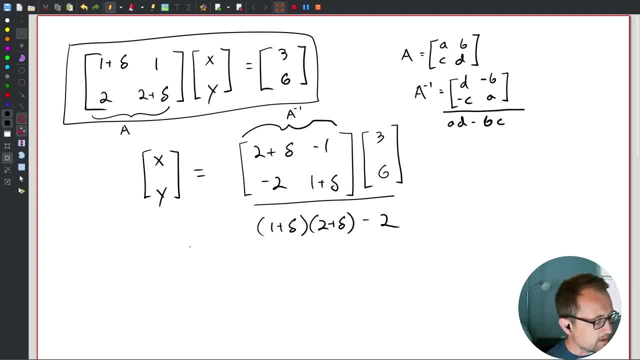 So that's what I'm doing here. I'm taking the inverse and dividing through by that. So now my solution for X and Y, Y is going to be- I'll just turn this into the vector- So 3 times 2 plus delta minus 6.. 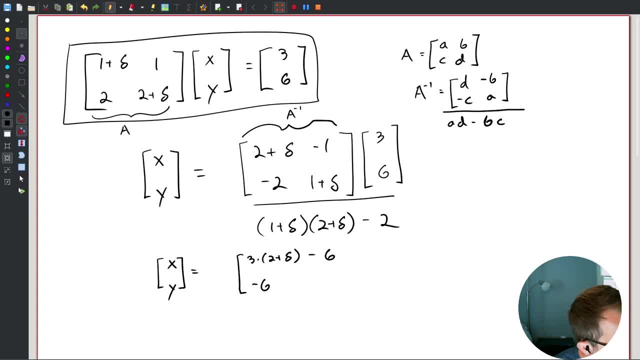 And then negative 6.. Take this 2 times that, 3. The negative 2 times 3.. Plus this 6 times 1 plus delta, And all of that is divided by This delta times. This should be a 3 plus delta. 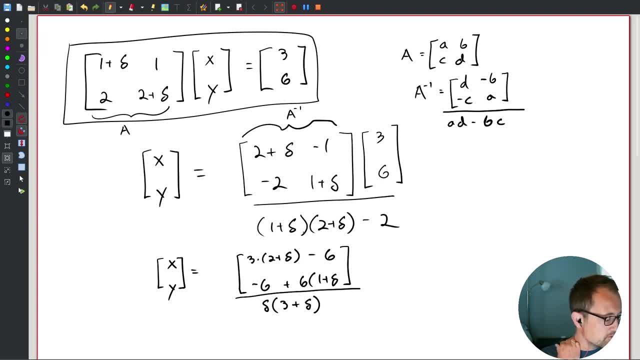 Like that: Factoring this out. there's a 2, there's a 3 times delta And then a delta squared term Factoring all that out. So the 2 cancels with that 2.. We just have this final value there. 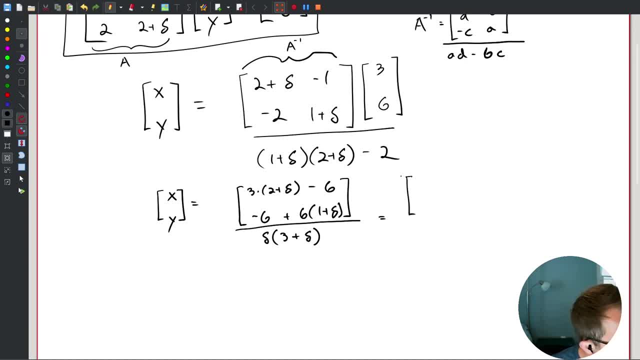 These 6's all cancel out. So I have a positive 6 and a negative 6.. So I'm just left with 3 times delta up top, And on the bottom the 6's cancel out again And I'm left with 6 times delta. 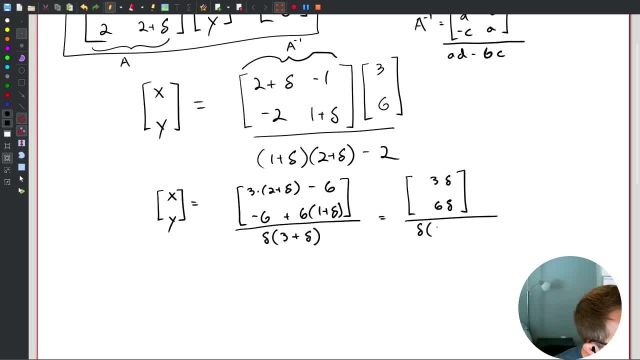 And again all divided by that, delta times 3 plus delta. So X is going to be 3 delta, 3 delta over delta, 3 plus delta, Or 3 over 3 plus delta, And Y is going to be 6 delta over delta times 3 plus delta. 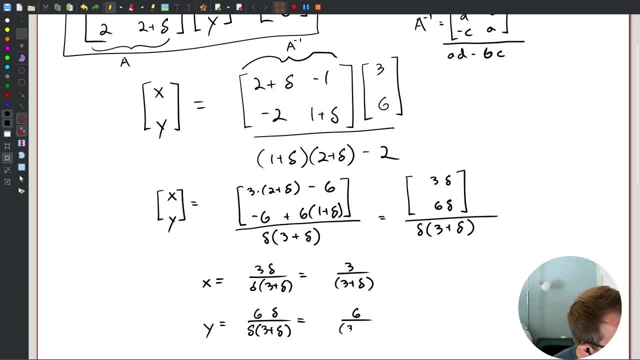 Or 6 over 3 plus delta. If delta is really small- If it's exactly 0,, then this becomes 1.. And if delta is really small here, this becomes 2.. So it's an exact answer, But the condition number in this case is: 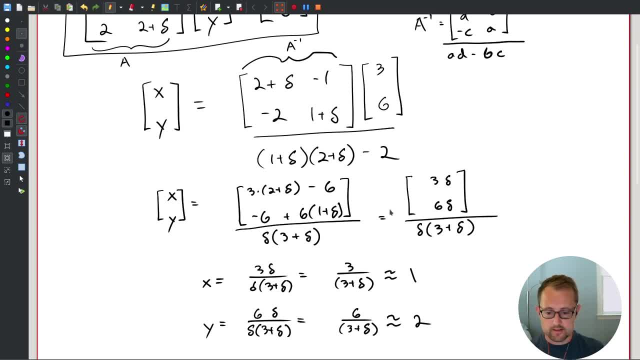 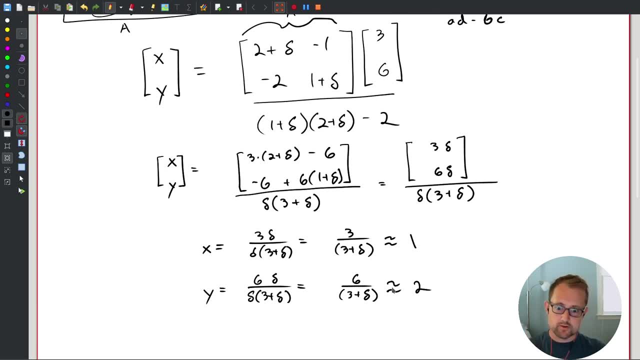 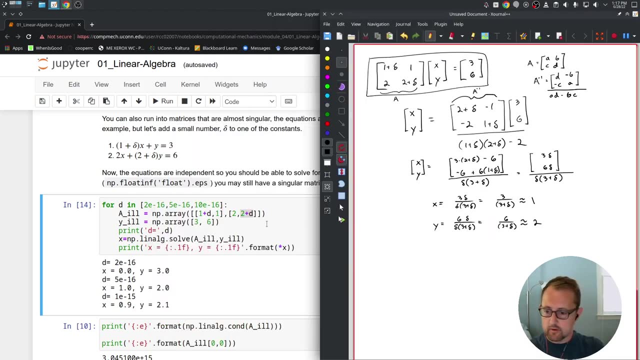 Because I can only store it with those. I can only store with 64-bit floating point. I have a large condition number And I'm going to introduce error when I try to solve this with a computer. So this is the answer that I'm looking for. 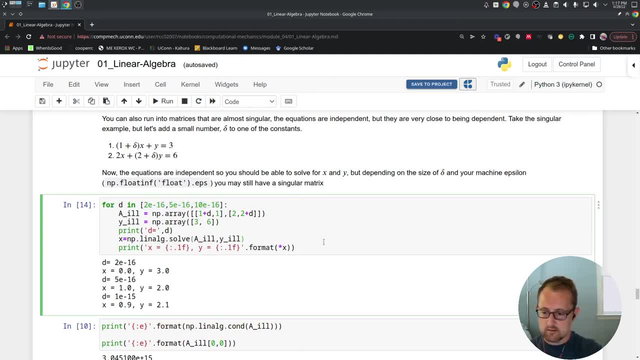 And depending on what these values are, Sometimes X is 0.. Other times X is 1.. Sometimes it's 0.9.. But it's changing by just a little bit And I can change these to. We could even try something else. 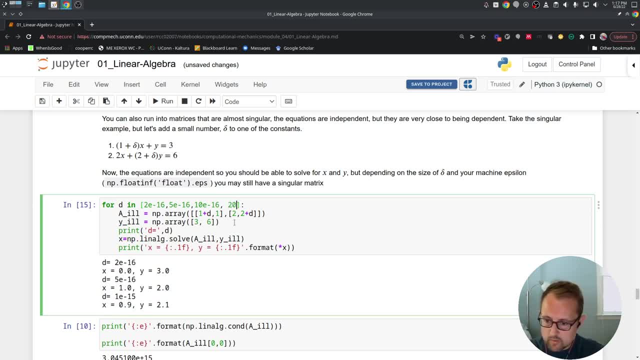 Let's do like 20.. Yeah, let's say like 10E to the negative 12. And then we actually get the right answer: 1 and 2. Which is what we got for 5 times 10 to the negative 16.. 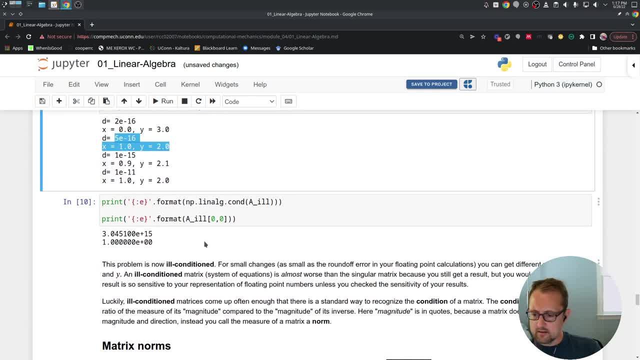 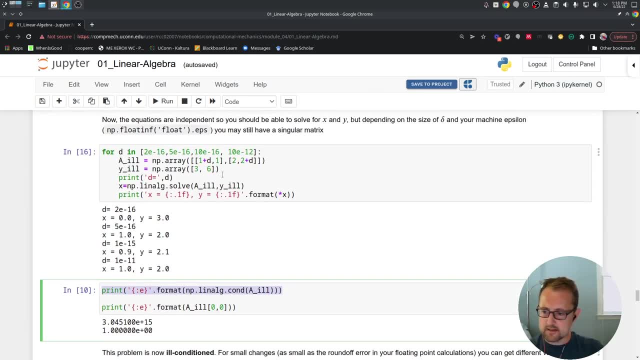 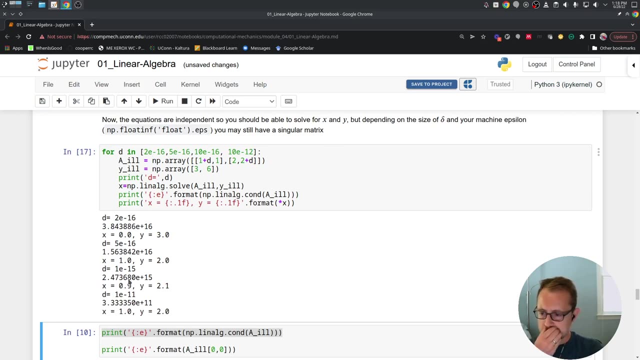 And the key here is that the condition Is figuring out what that condition number is And that tells us, like, How much error there is here. So let's add that print statement in here. The condition number here Is some power of 10 to the 16.. 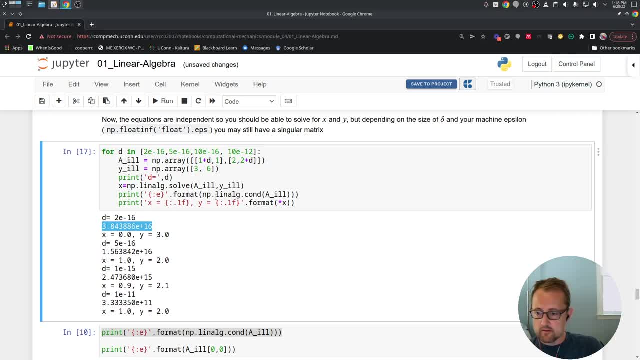 And the. The best case scenario is that I can store numbers with accuracy of 10 to the negative 16.. That's my float, That's my machine epsilon term. So I'm going to have error On the order of 1.. 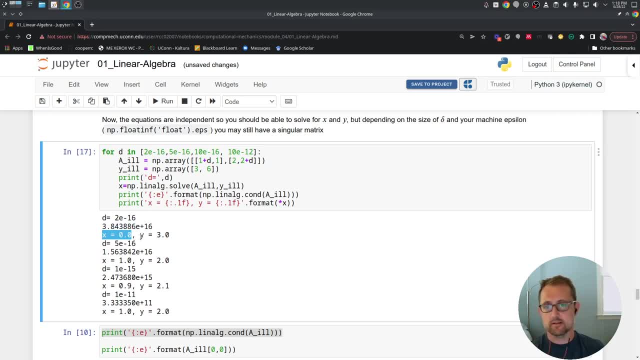 Which makes sense that The actual answer is 1.. But I solve for 0.. And here the actual answer is 2. But I'm solving for 3.. So it's So the This answer, 3, is really 3 plus or minus 1.. 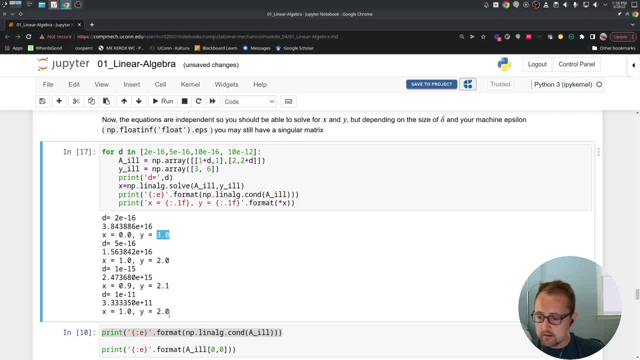 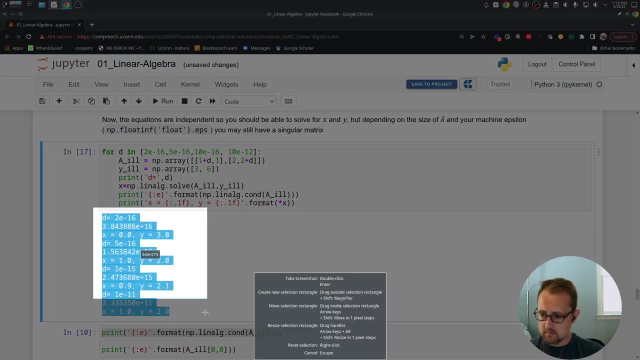 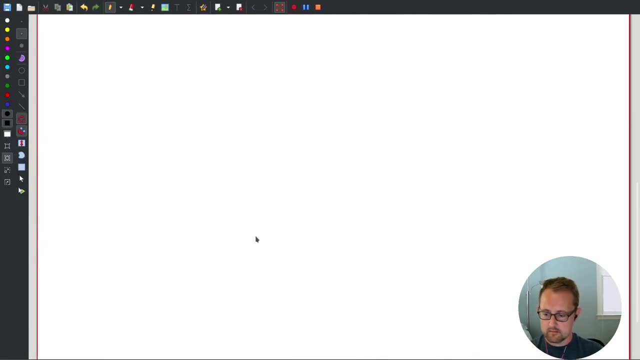 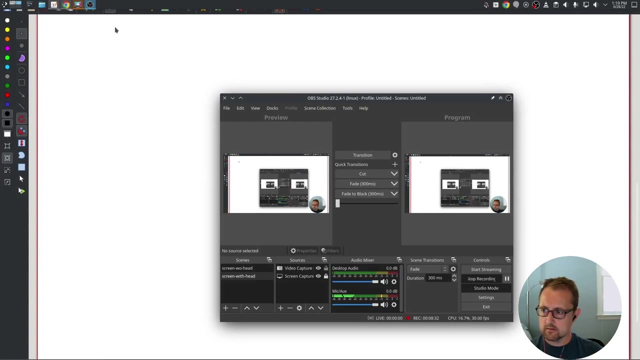 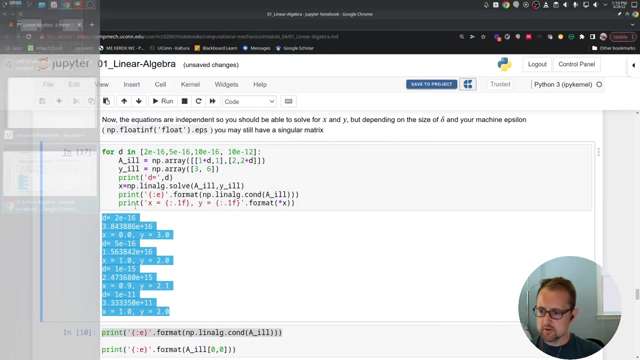 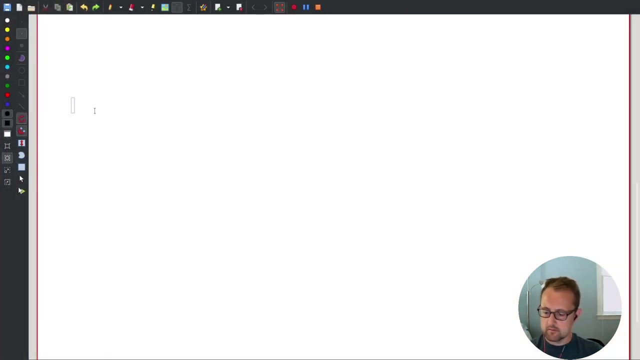 Because it's 10 to the 16.. Let's copy these over. Ah, Let's take that And bring it over here. Oh, I'm just trying to Trying to get this stuff over there. There we go, So the error. 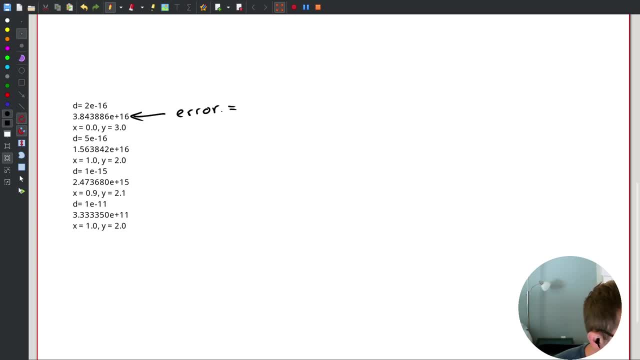 For this condition number, The expected error is going to be 10 to the 16 minus 16. Which is 10 to the 0. Or 1.. So these two answers Are 0 plus minus 1. And 3 plus minus 1.. 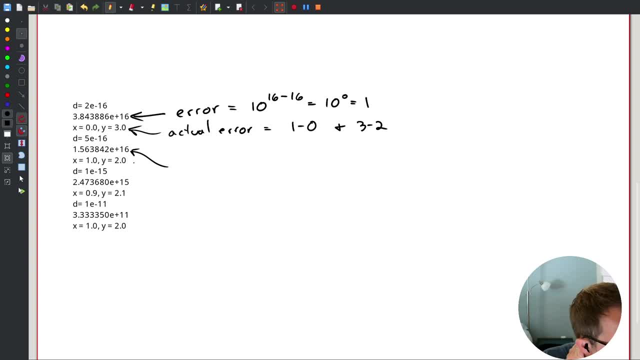 In this case, Again, the error is 10 to the 16 minus 16. Which is 10 to the 0. Which is 1 again, But Here we actually have The actual error is 0. Because it's solving for the correct values. 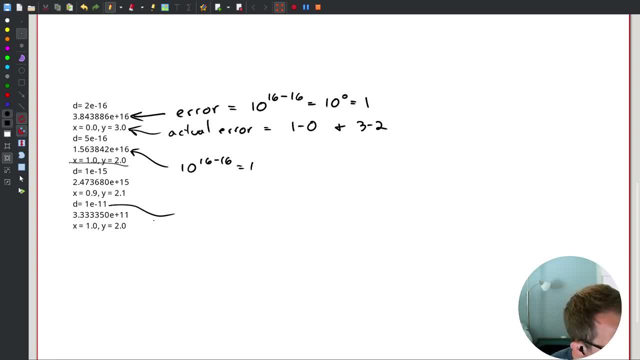 Now let's Compare that down here. Ah, Not that one. My error Is 10 to the 11 minus 16.. The condition number is 3 times 10 to the 11.. So the only thing I really care about. 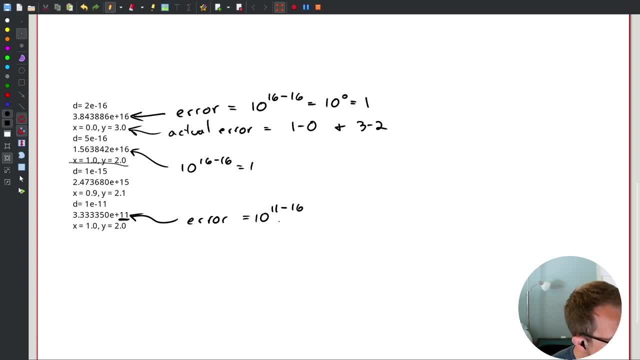 Is that power, How big it is. So it's 11.. 10 to the 11 minus 16.. Or 10 to the negative 4 error, Which is really small. And that makes sense, Because this is The actual error there. 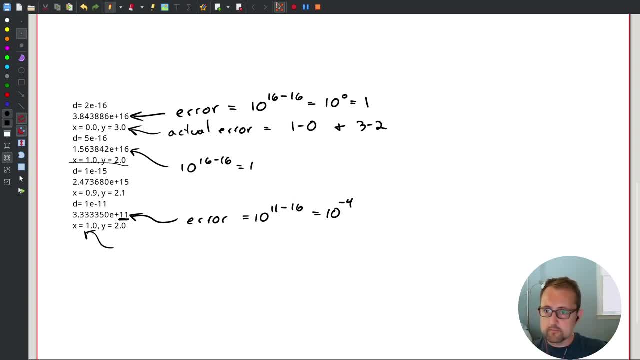 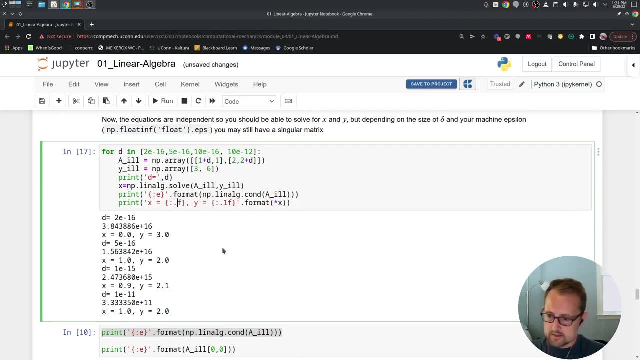 Is Probably about 10 to the negative 4.. Let's take a look, Let's turn this into Maybe 9 significant figures. Yeah, So it looks pretty good so far. Maybe 25.. Now we can start to see. 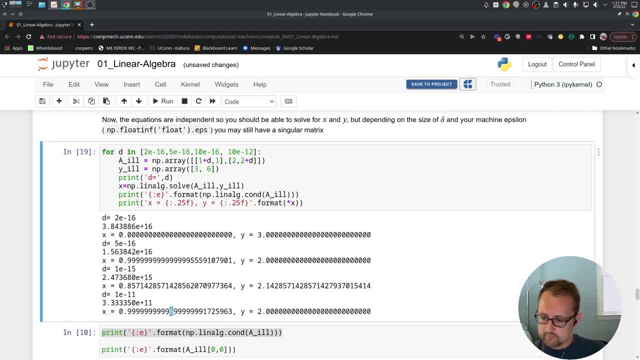 A difference Out here In the 1,, 2,, 3,, 4,, 5,, 6,, 7,, 8,, 9,, 10, 11th Decimal place for x. So even that is. 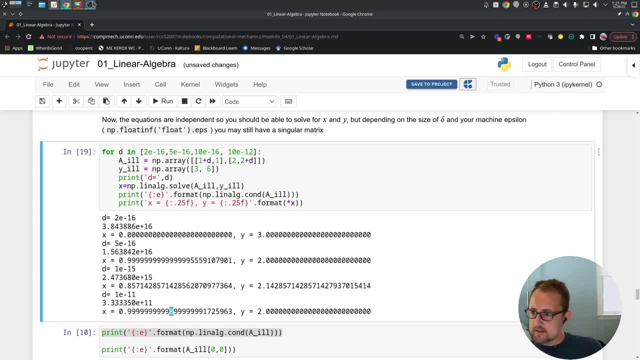 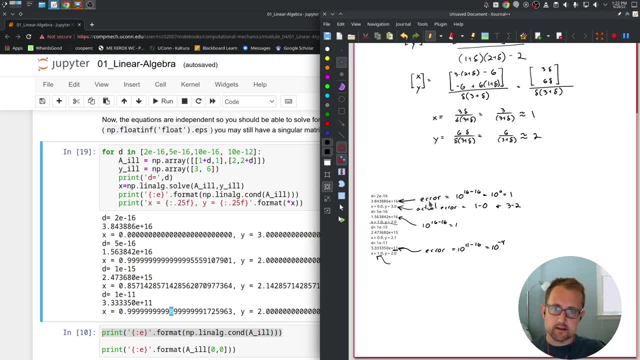 Is closer Than the error. This error that I'm calculating, In this case The. This is the, The worst case scenario, Like the worst error that we can have Because of Combining floating point operation errors, High condition number. 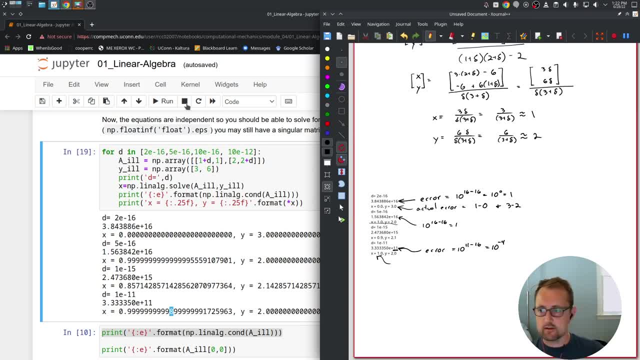 Means less accuracy When you're actually trying to solve that problem. This is: This is kind of a This is kind of a cool concept. I think it's a cool concept Because it shows you what the limits are And the number of times that I've gotten.